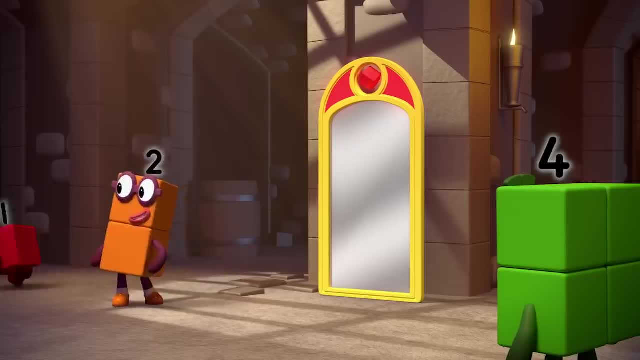 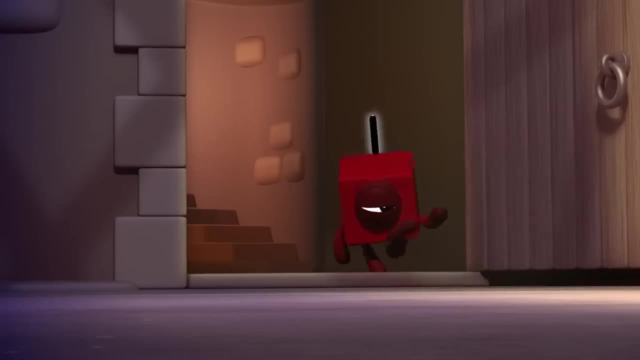 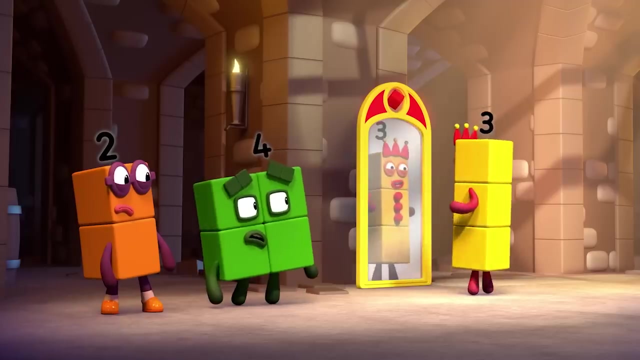 The others will want to see this. Keep an eye on it while I'm away and don't mess around with it. Right, My turn. One said not to. Oh, Go on, It's only fair. Two lots please. 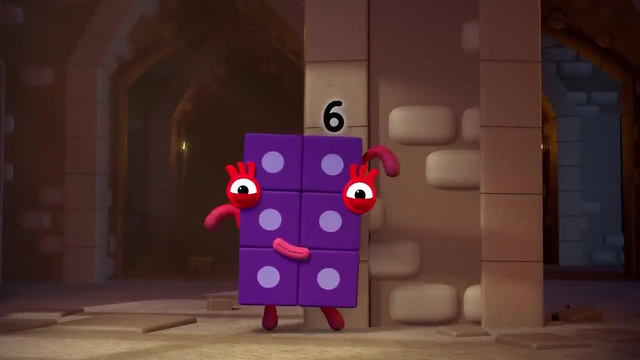 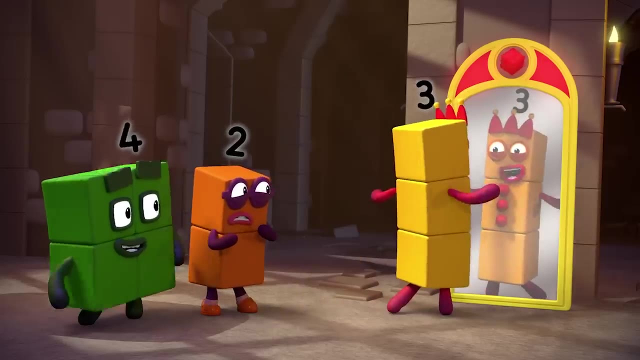 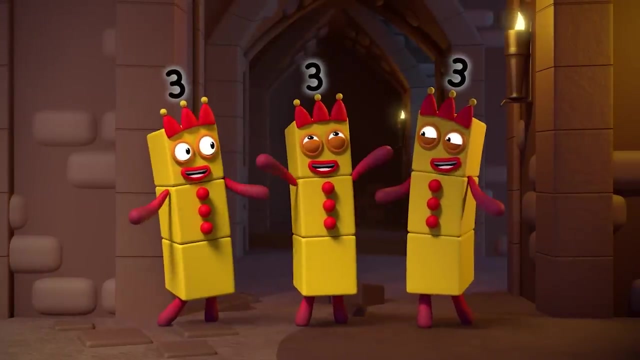 Two lots of three is six. Number six is on the floor. Don't be shy, let's have some more Good idea. Three lots, please. Three lots of three is nine And three- threes, see Ha Yay. 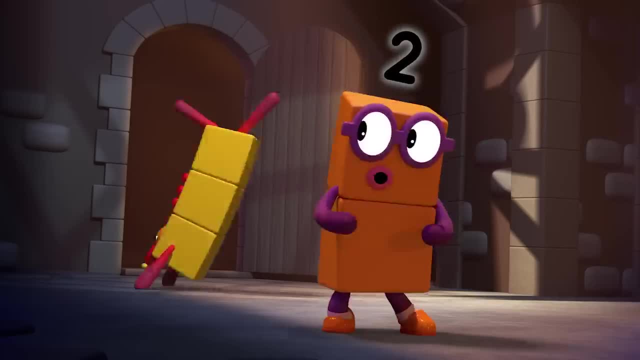 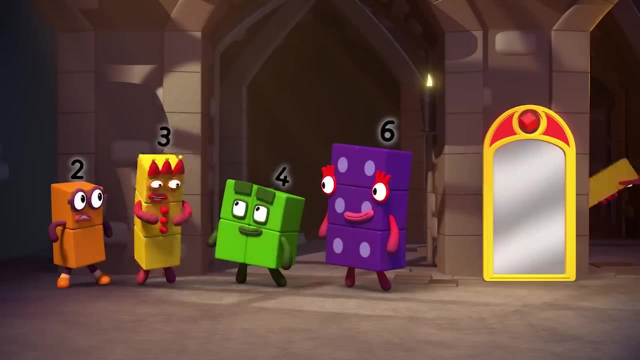 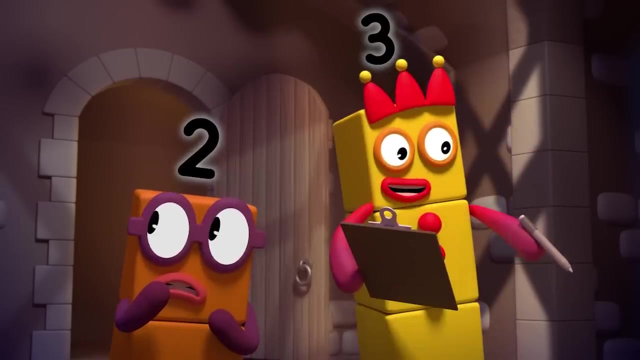 Oh yeah, We should probably stop now. But look, there are so many of us here already. What would be surprised if she comes back and everyone's here. All right, then We've got two, three, four, then six. 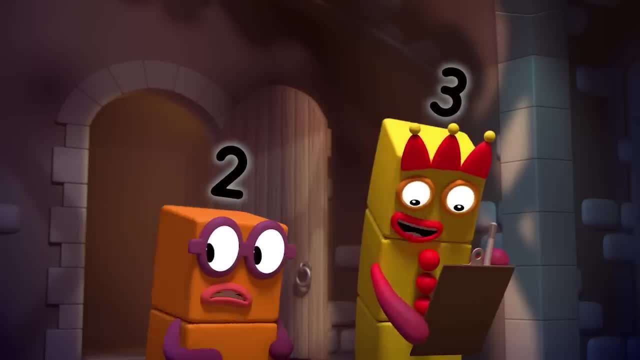 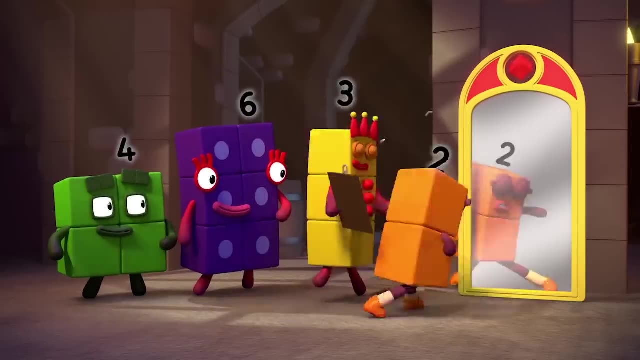 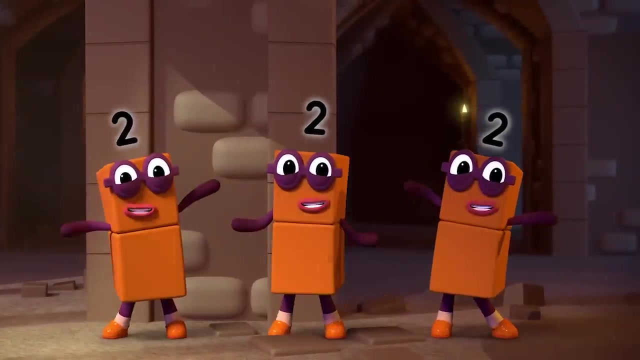 Oh no, We're missing five. How many lots of who is five? Hmm, let's try you. Oh, Three lots, please. Three lots of two is six. Number six is on the floor. Wait, have I said that before? 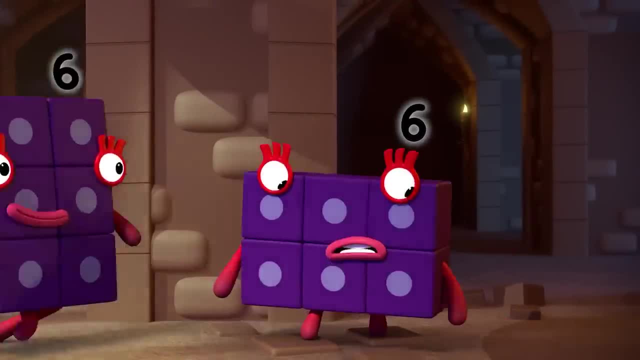 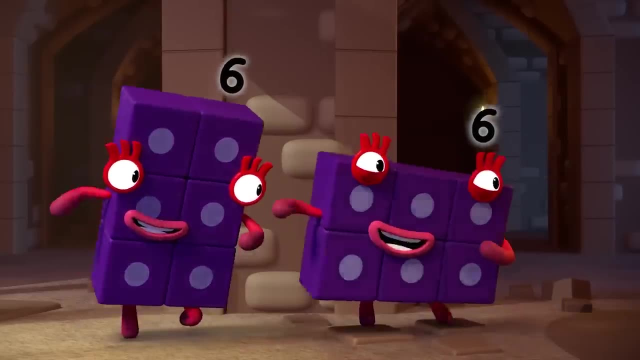 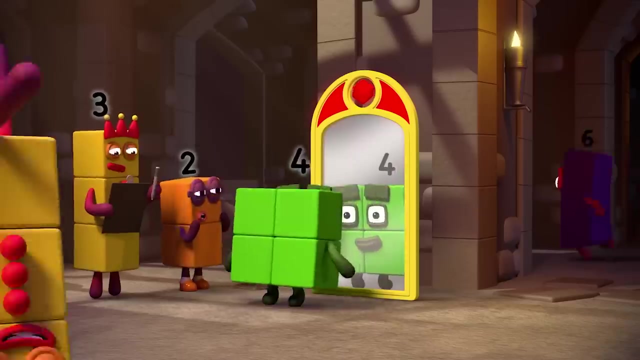 Two lots of three. Three lots of two, Ha Ha Ha. Yay, I was hoping for a five. Maybe I can help. No Two lots, please. Oh. Two lots of four is eight, Oh yes. 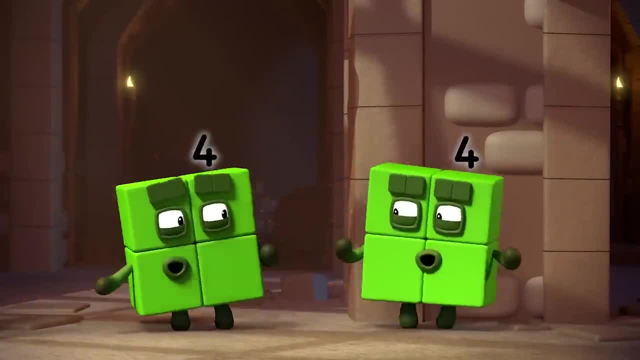 Two lots of four is eight. Oh yes, Three lots of two is eight. No, no, no, We need a five And we're missing seven and ten. Who wants to try next? Oh, It's a big surprise. 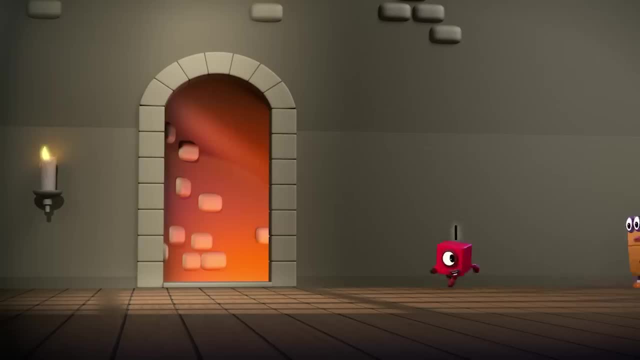 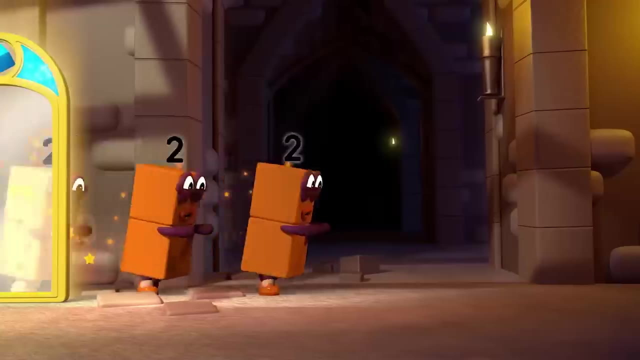 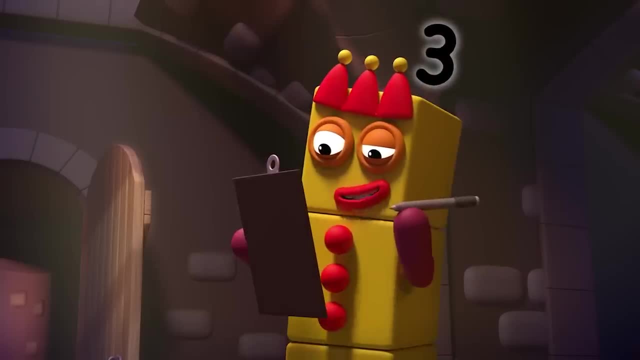 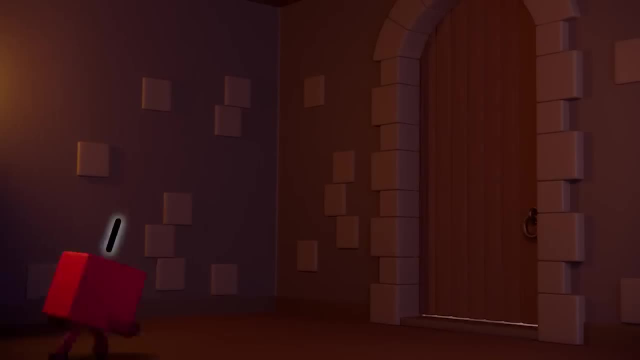 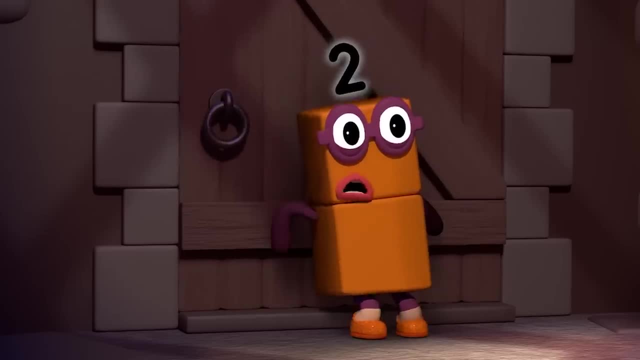 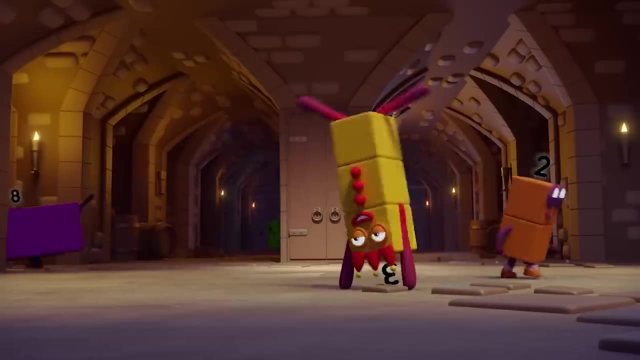 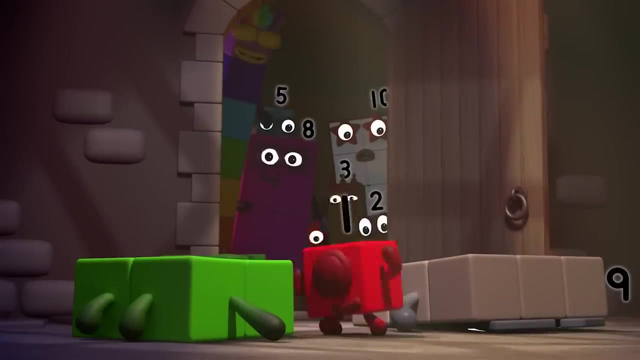 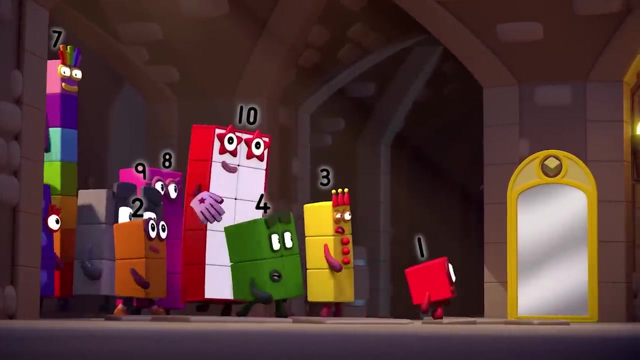 Onunca, Agora One's coming Hide, Hide. Why can't we make five and seven There? Surprise, Oh, A magic mirror, Pretty Looky-cook, Ah. but what if I said I could make lots of number blocks appear all at once? 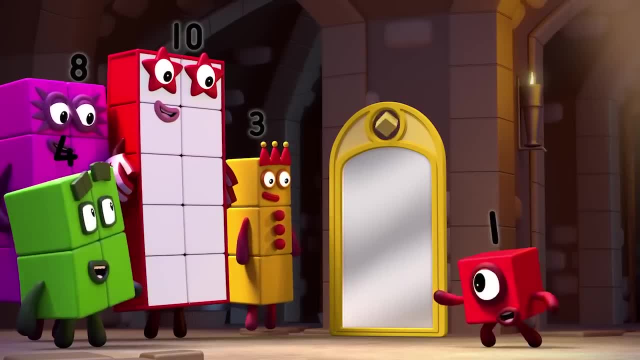 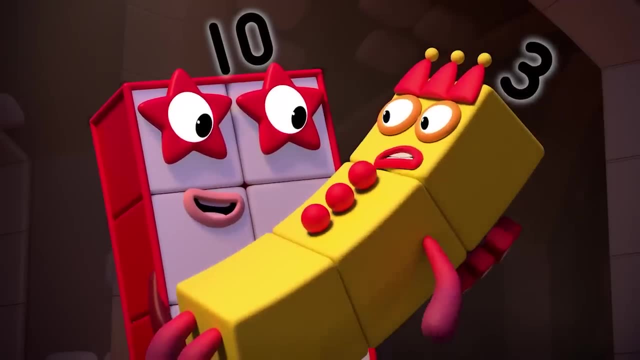 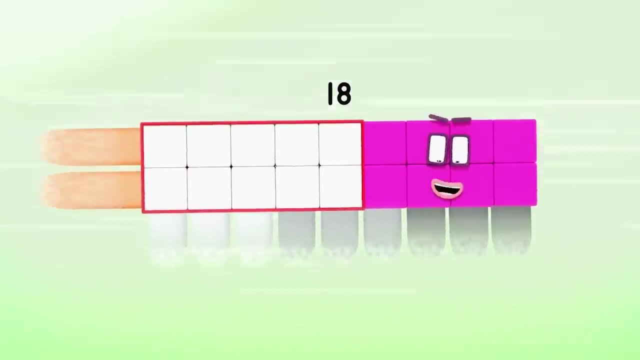 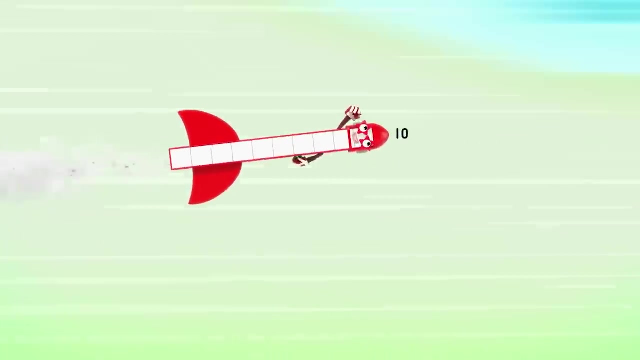 Now that would be a Surprise. Woo-hoo, Here I come. I need more speed Switch three rays and away. Woo-hoo, Hooray. Six, nine, twelve, fifteen, eighteen, Huh, Oopsy. 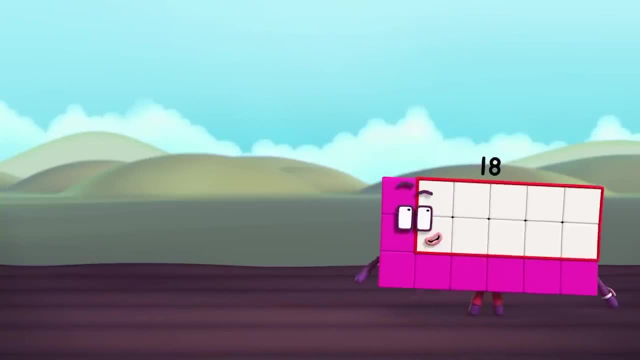 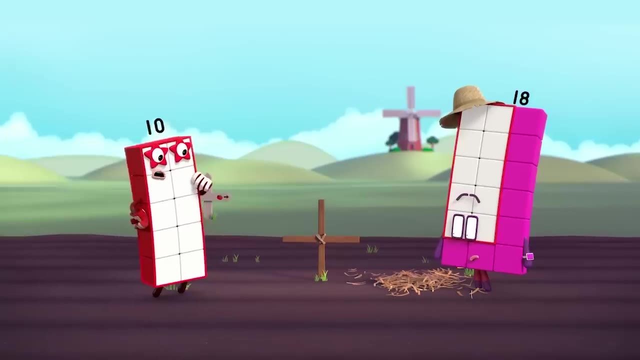 You know, I'm sure there was an old scarecrow here, Scarecrow No. Can't see any old scarecrow, Just uh, I don't know. I'm sure there was an old scarecrow here, Scarecrow No. 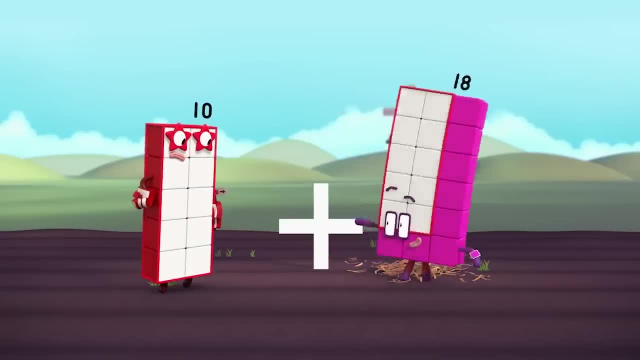 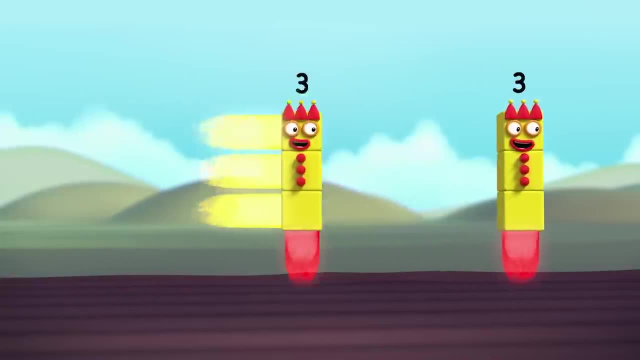 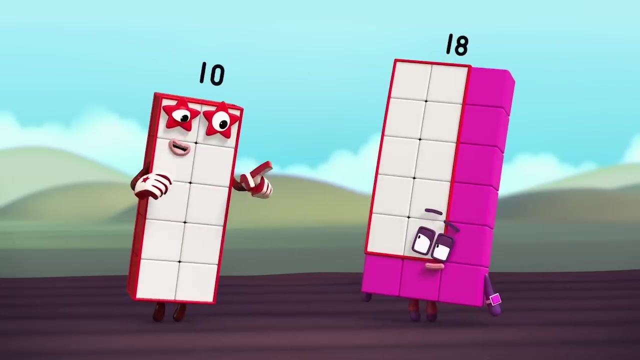 Just this great big plus sign. Hey, we can use it to practise adding up really fast. Oh, Three, six, nine, twelve, fifteen, eighteen. I love that trick. Could you slow it down so I can see how it's done? 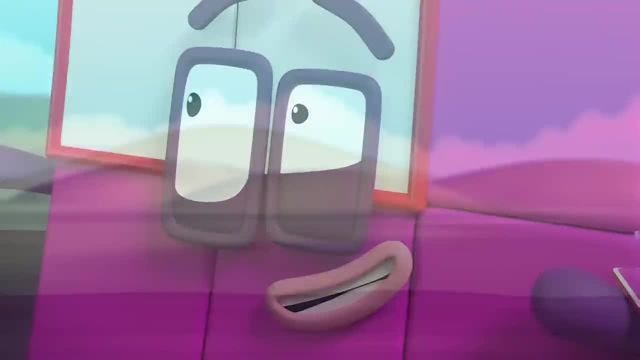 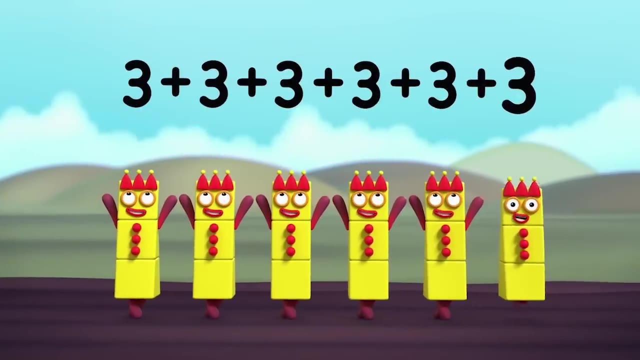 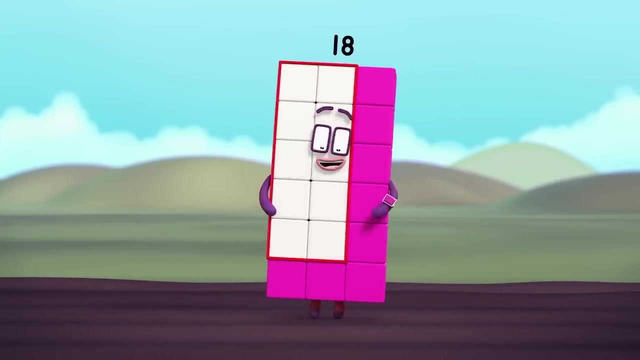 Well, just this once On your marks. check Three, three, three, three, three, three, three Equals three. Six, nine, twelve, fifteen, eighteen. Slow enough for you, I'm just adding three. lots of times. 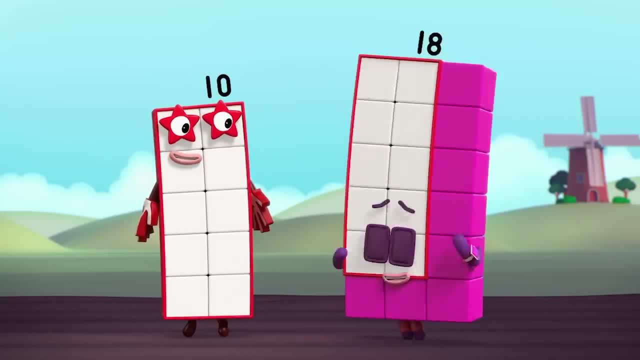 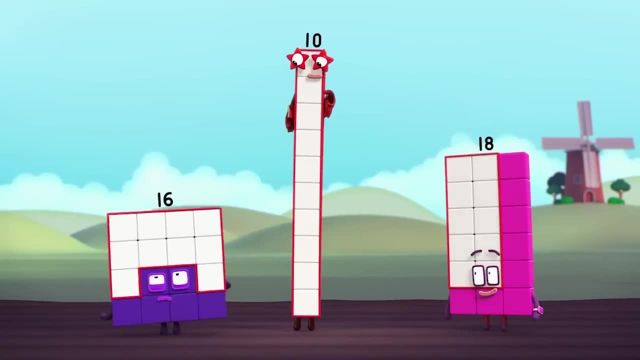 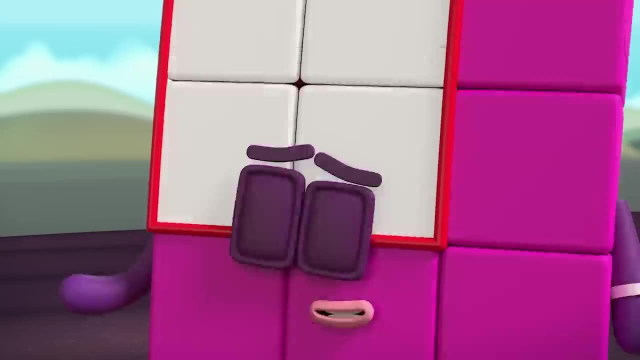 The trick is to know how many times Try it. Ten Um, All right, my friends, I've come to pan some square potatoes. Imagine the chips. Hey, where's the old scarecrow gone? So Ten ready yet. 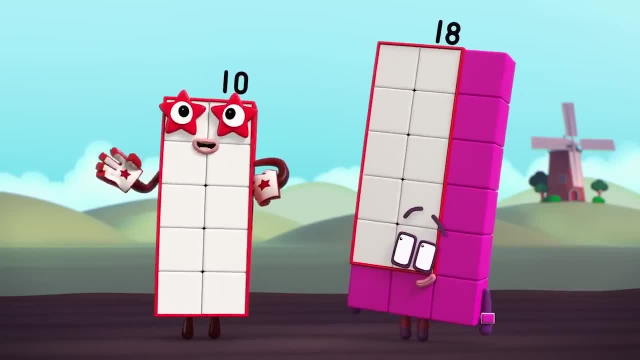 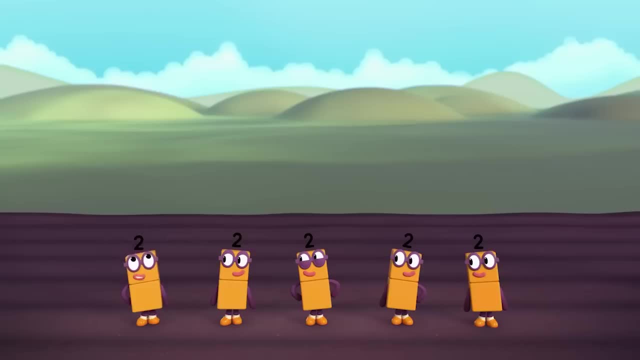 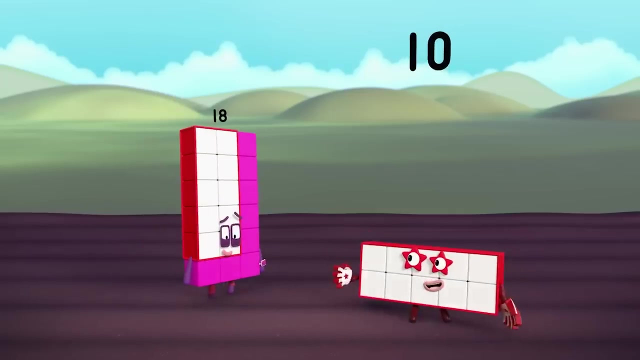 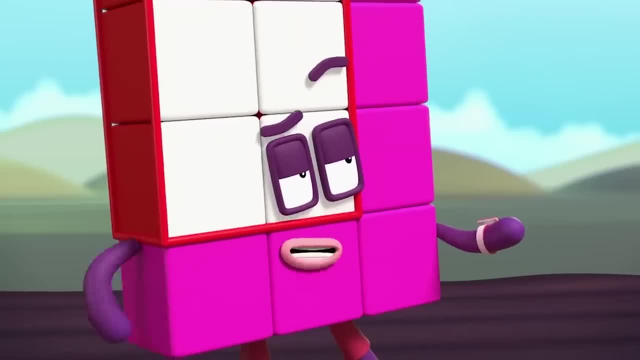 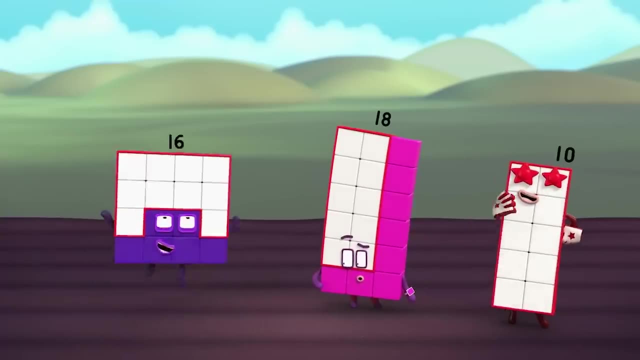 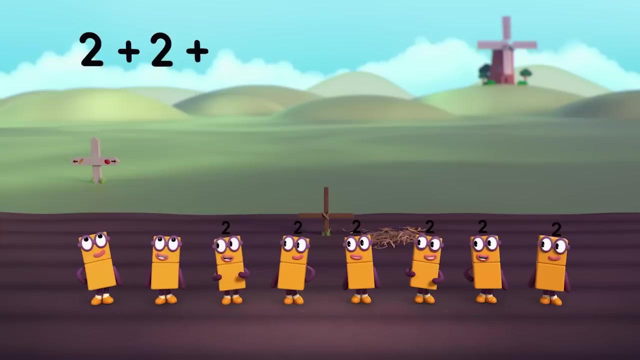 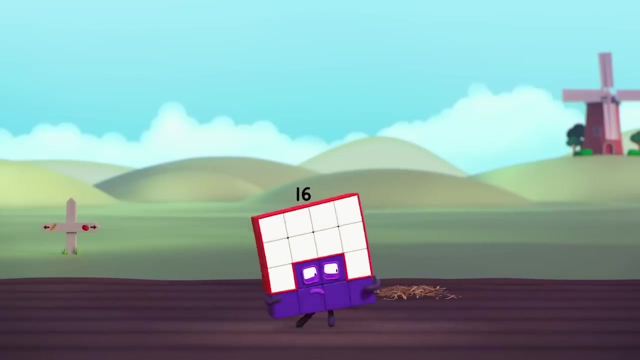 We got there in the end, But did you have to go so slow? You like it fast? Let me have a go. You would believe your eyes. Two plus two plus two- Argh, This is gonna take all day. I'm sorry, Eighteen, but you made me lose count. 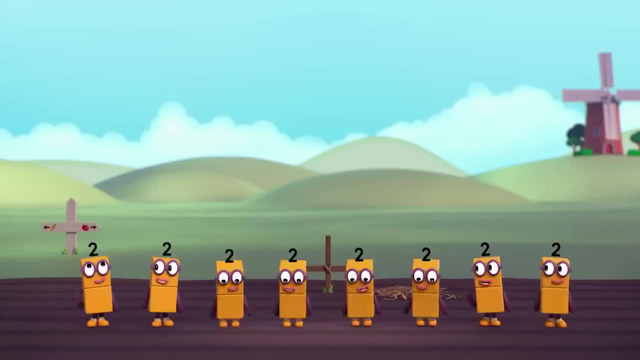 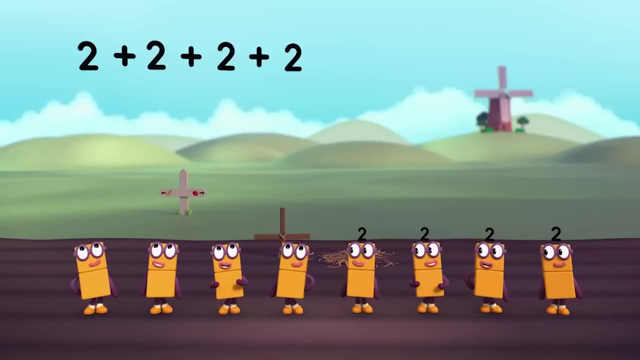 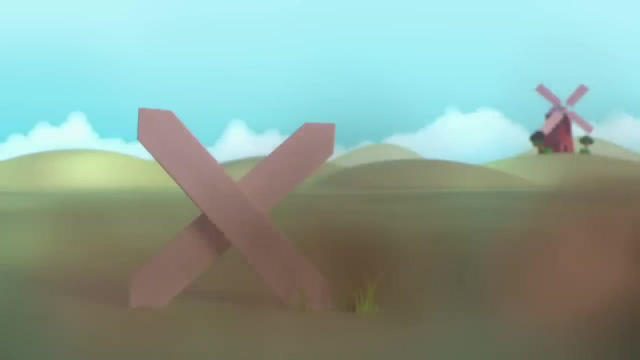 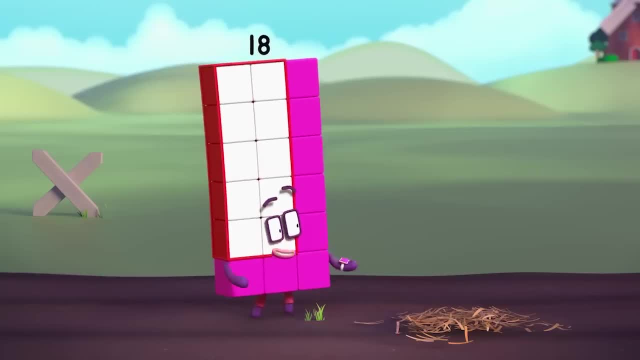 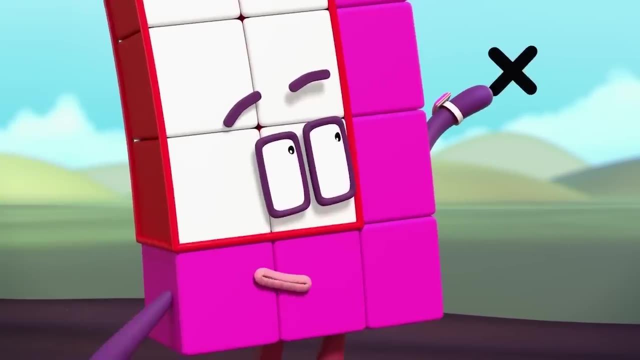 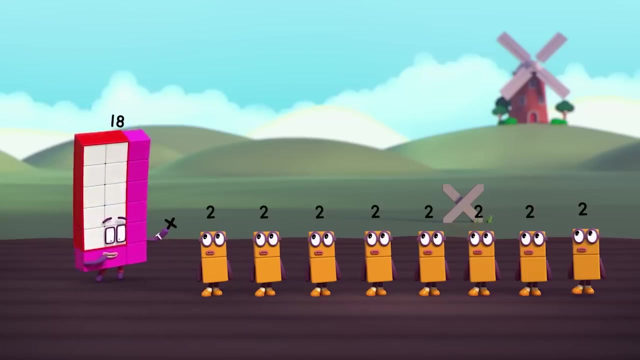 A sign that we need a new sign, A faster sign. We don't need all these Squash. we can add a number lots of times, Much faster with just one of these. I'll call it the times sign. I can use it to add something lots of times. 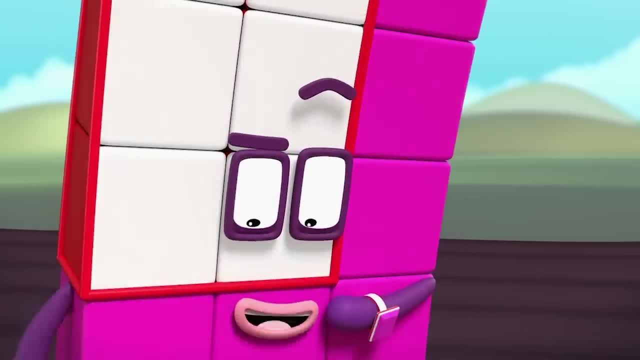 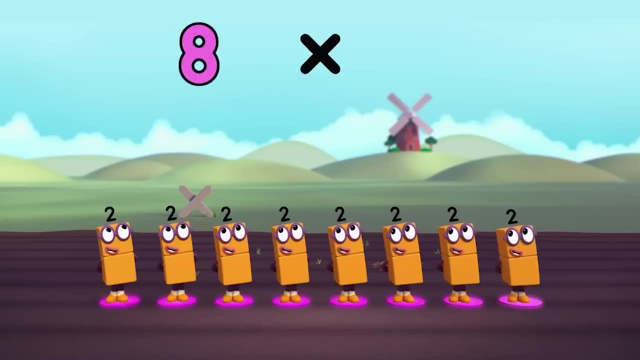 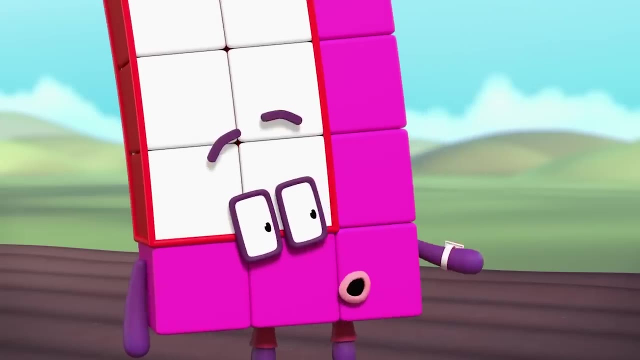 Super quickly. So how many twos are we adding? One, two, three, four, five, six, seven, eight. And remind me, what are we adding again? Twos, Eight, lots of two. On your marks, get set go. 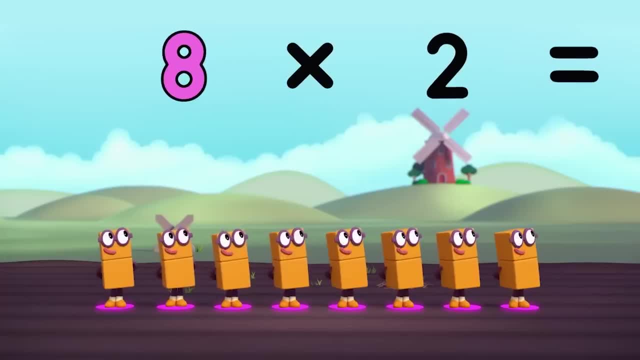 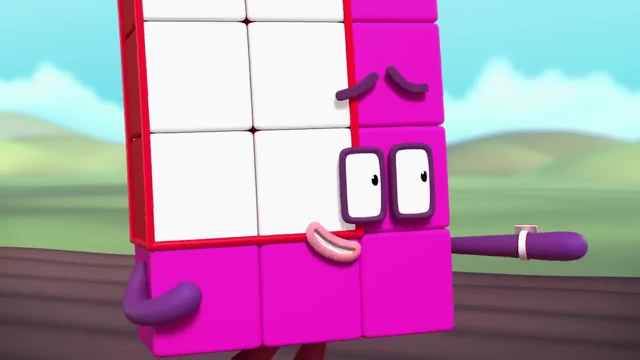 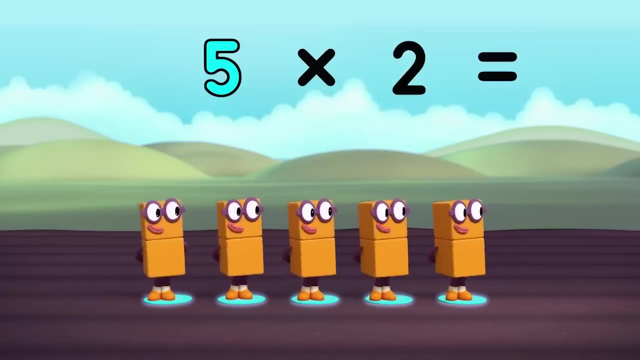 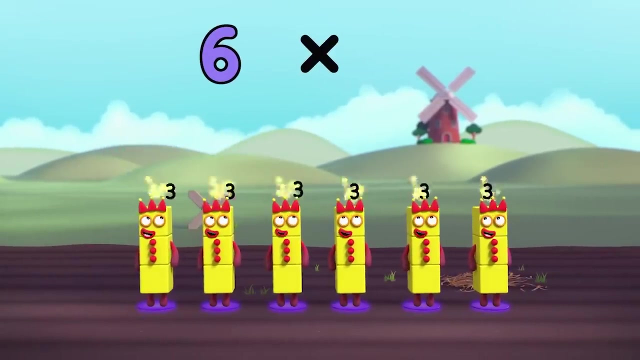 Eight times two equals Sixteen, So much faster. Ten. go again On your marks. There are five of us. Five times two equals Ten On your marks. get set: go. Eight times two equals Eighteen. 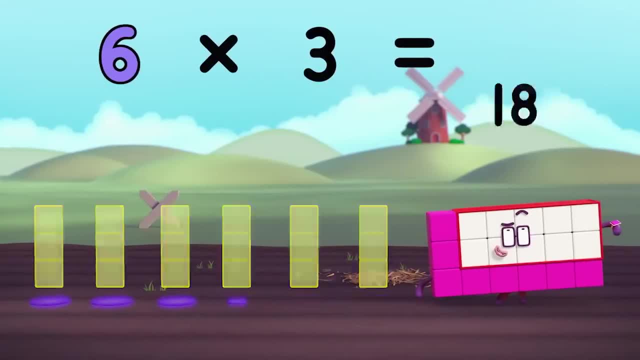 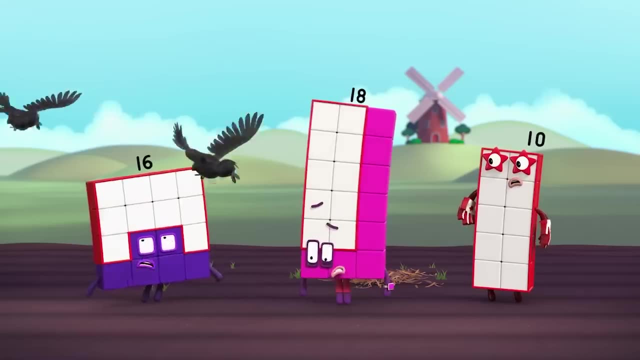 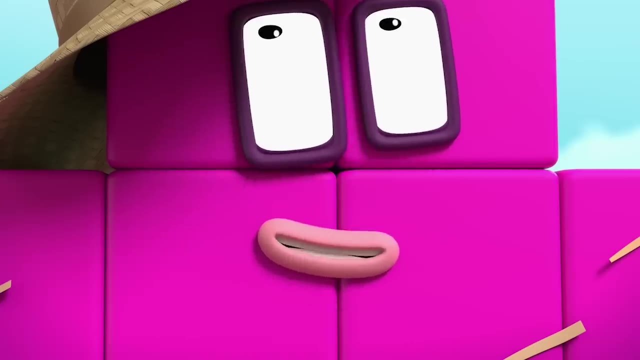 Six times three equals Eighteen. Refreshingly fast, This makes up for breaking some silly old scarecrow. Whoops, Ah, Eighteen, Eighteen, No, I can't see any eighteen, Just this good old scarecrow, Ha-ha-ha. 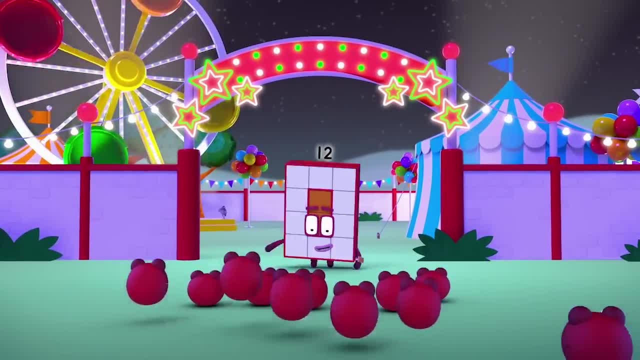 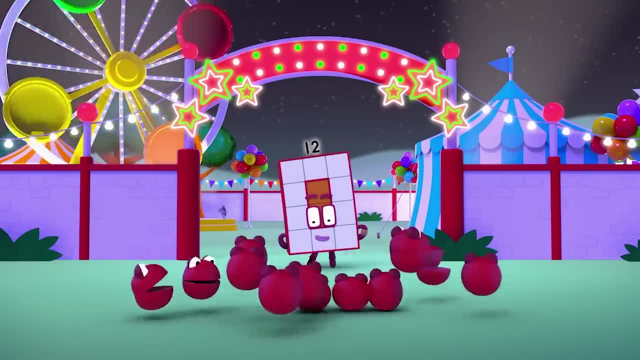 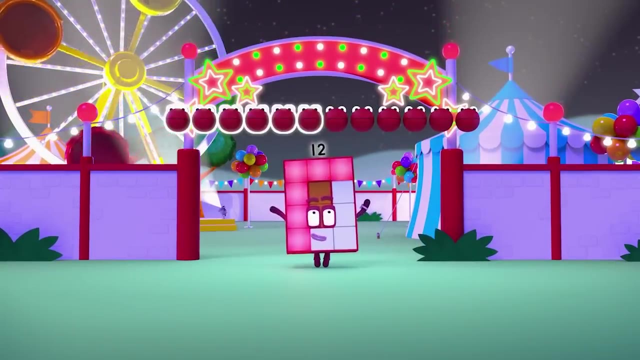 Welcome to the Fun Times Fair. Is everyone here? Yay, One, two, three, One two. Oh, come here. One, two, three, four, five, six, seven, eight, nine, ten, eleven, twelve. 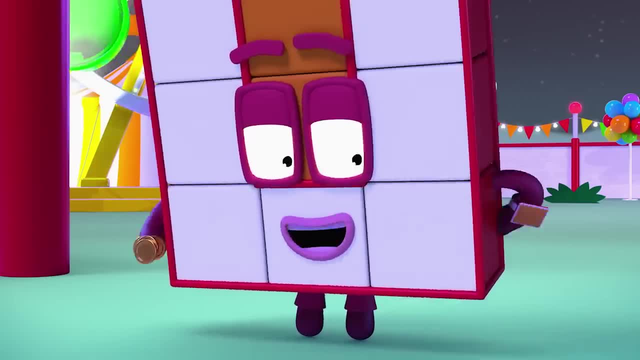 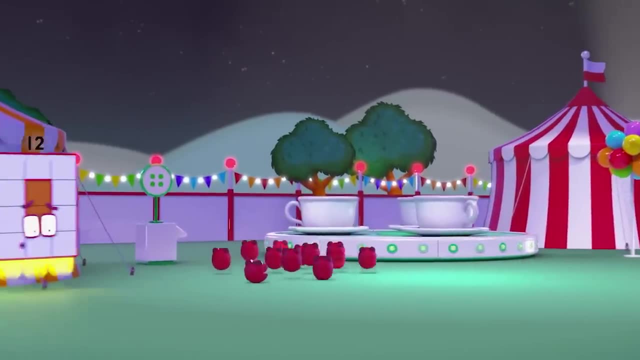 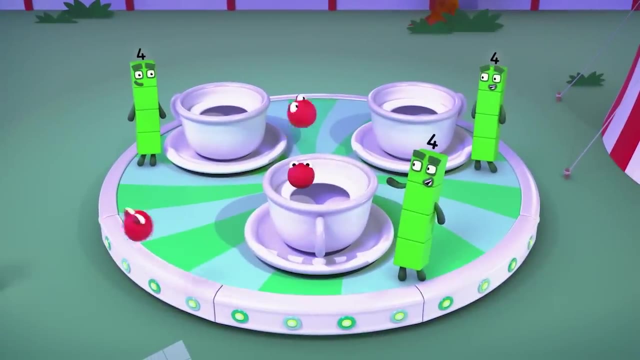 Twelve number blobs. Good, I've got lots of ride tokens. What would you like to The teacups? The teacups, Hmm, It looks like four to a cup. Look One, two, three, four. One, two, three, four. 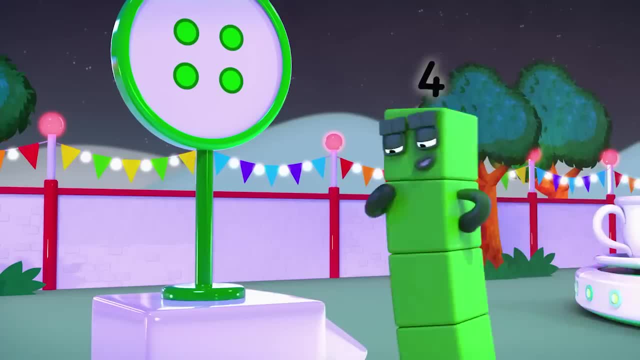 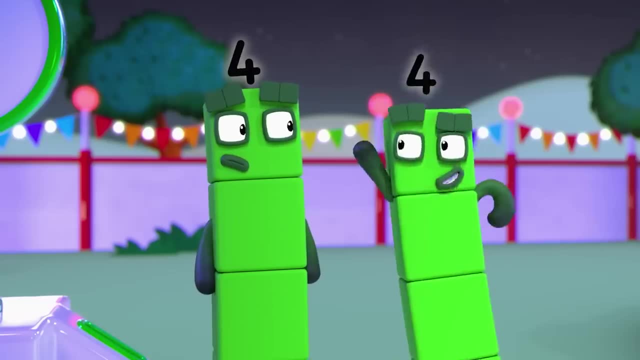 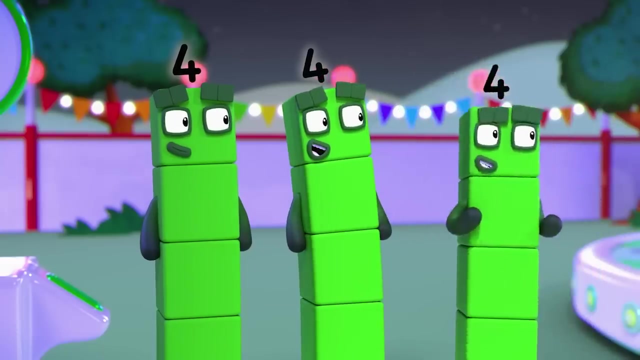 One, two, three, four, Ha-ha-ha. Now, how many ride tokens do you need? Um, Look at it this way: How many cups are there- One, two, three, Three cups- And how many riders in each cup? 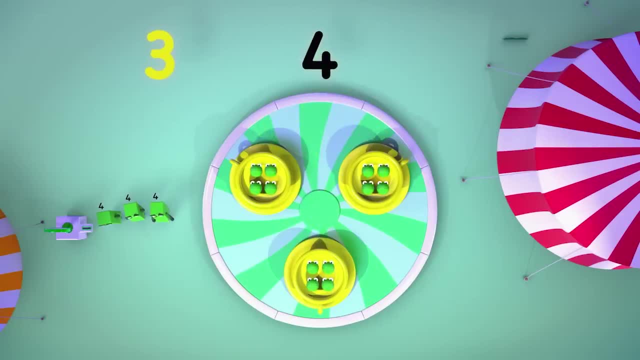 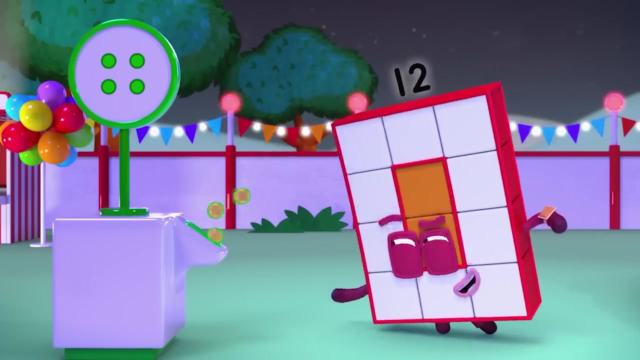 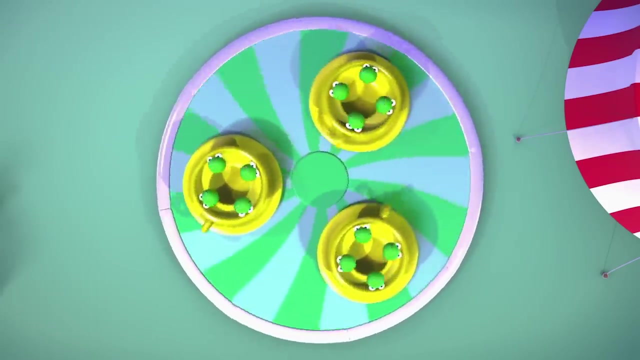 Four, So that's three lots of four. Three times four, which is Three times four, equals twelve. Three lots of four is twelve tokens, And off you go, Watch us spin. three lots of four, Twelve number blobs and not one more. 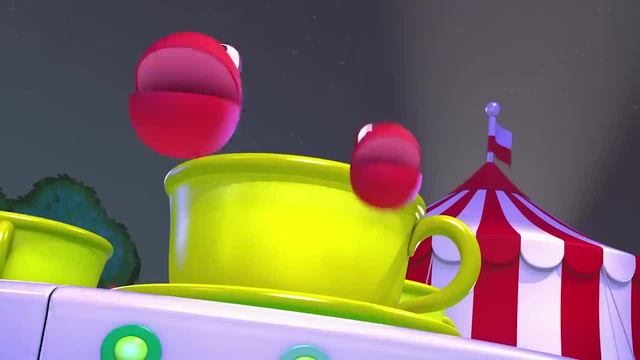 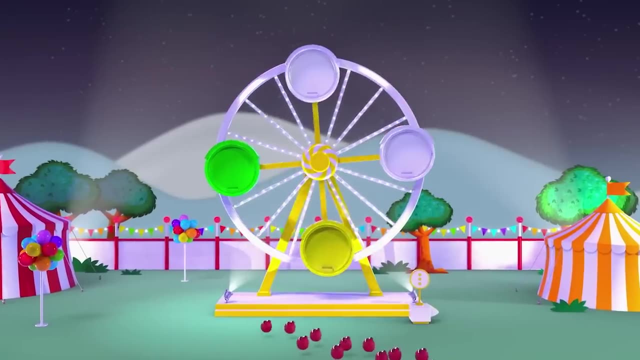 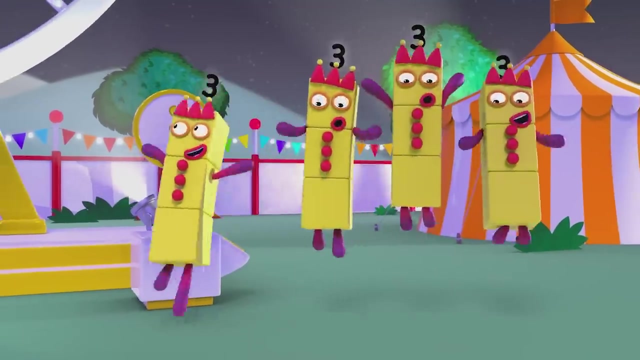 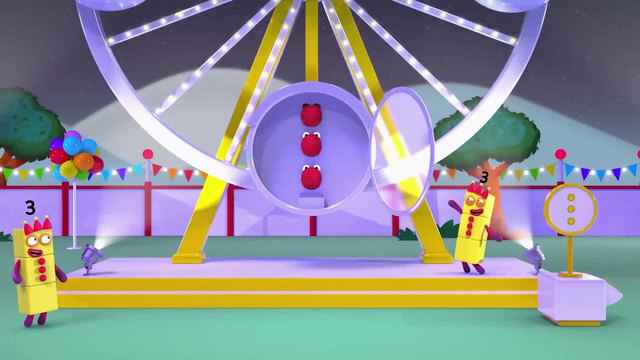 Whee, Ha-ha-ha, Ha-ha-ha. That was fun. So The big wheel, The big wheel, Aha, Looks like three to a carriage this time: Two, Three, Three, Three, Three. 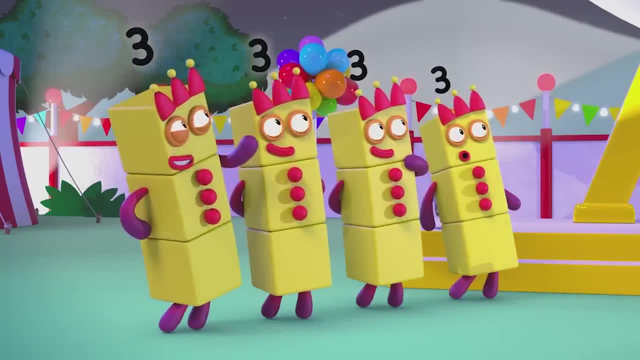 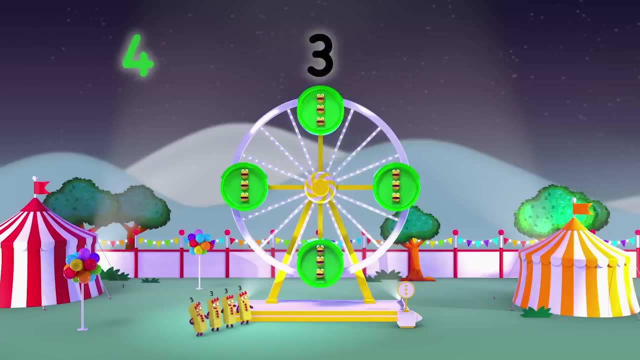 Time for tokens. How many carriages One, two, three, four, How many in each carriage? Three. So how many tokens do you need? Four times three equals twelve, Oh-oh-oh-oh-oh, Twelve tokens. 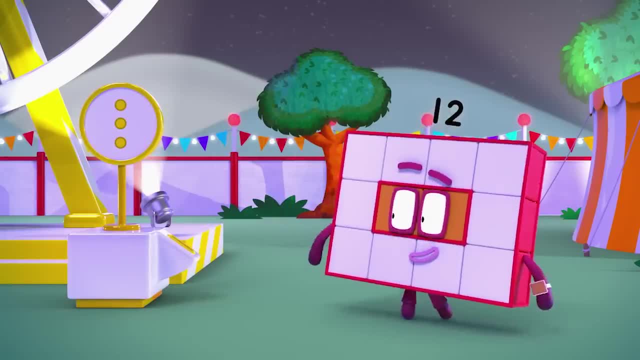 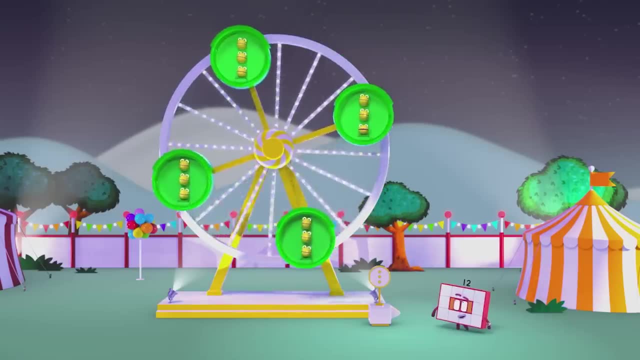 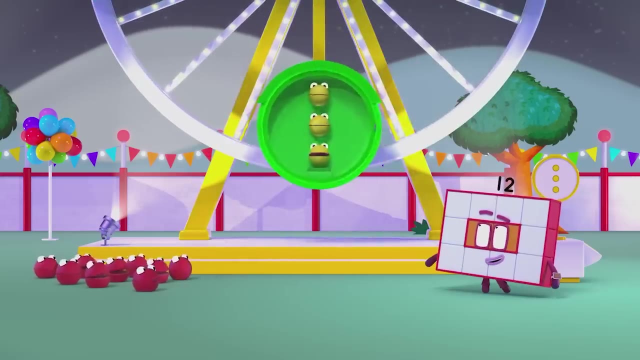 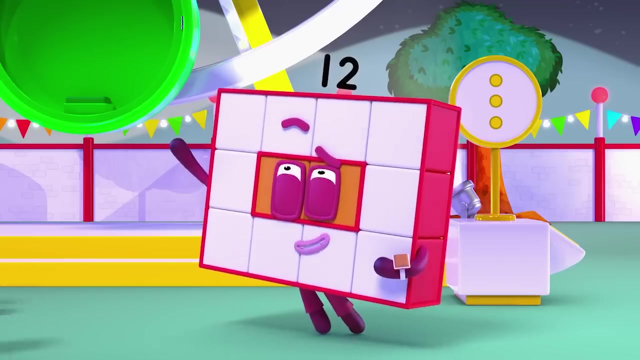 Four lots of three, Four lots of three. Around we go, Four groups of three, Twelve number blobs all going whee, Ha-ha-ha-ha, Ha-ha-ha-ha. Now, little ones, are you ready for the fastest, most thrilling most? 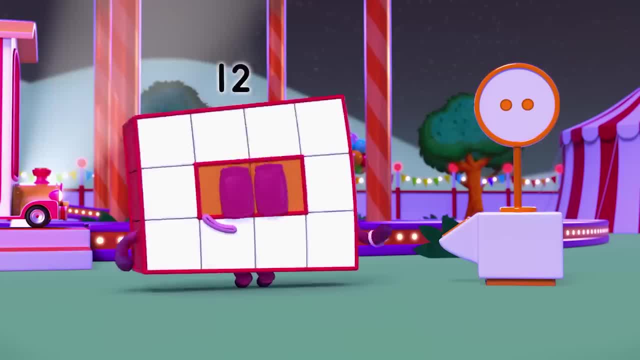 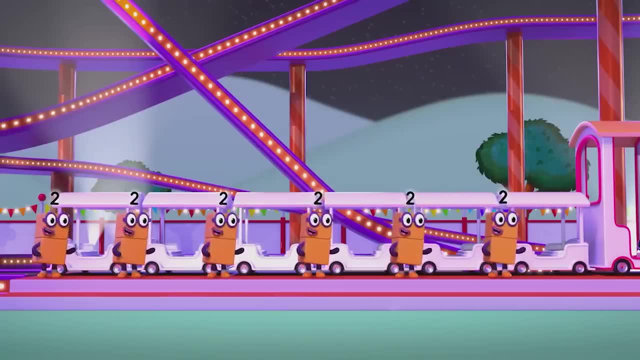 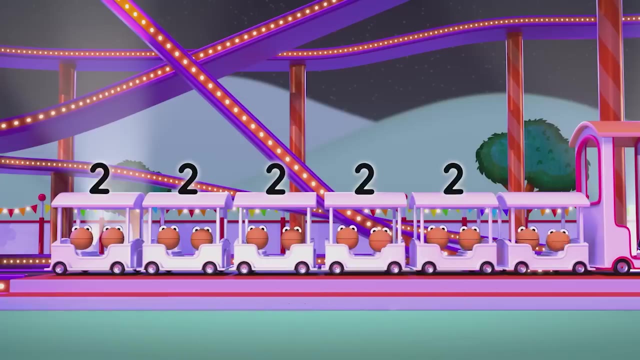 The Runaway Train, The Runaway Train, Hmm, Ha-ha In pairs, please Switch, Switch, All aboard. Two, two, two, two, two, two. Now, how many carriages are there? One, two, three, four, five, six. 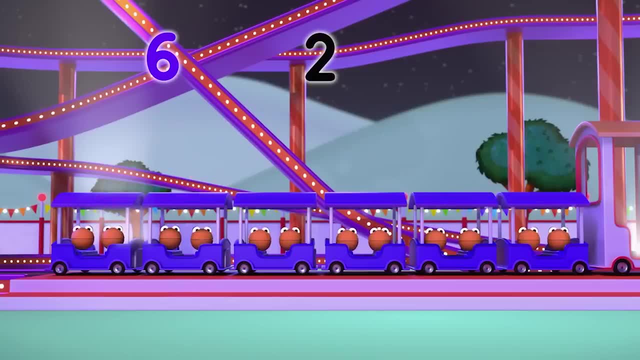 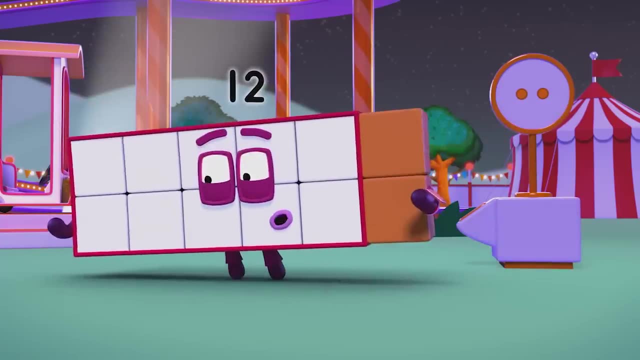 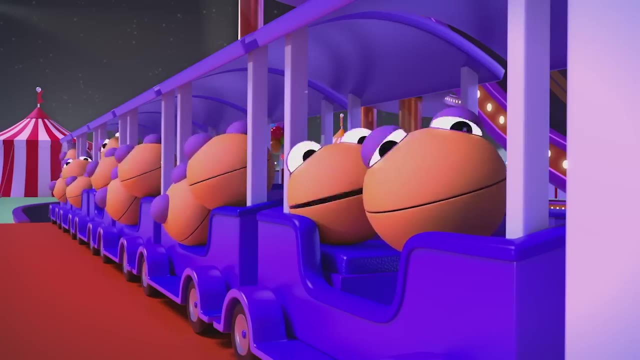 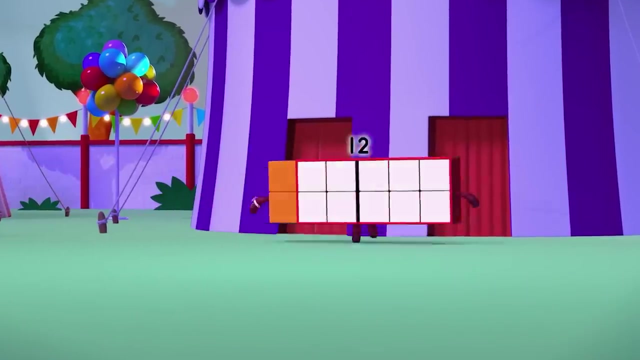 And how many in each carriage? Two, Six times two equals twelve, So you need twelve more. Oh, I'm all out of tokens. Oh, Oh, Roll up, roll up and have some fun. There's lots of tokens to be won. 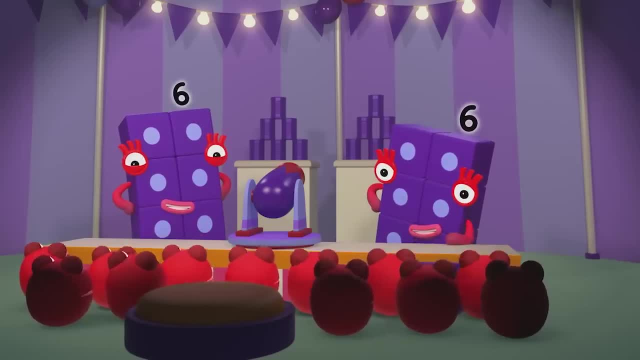 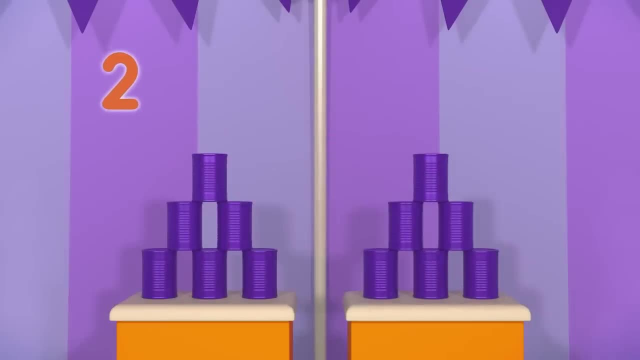 Oh, We need twelve tokens. You'll win one for each can that falls, and there's One, two, Two stacks. One, two, three, four, five, six, Six cans in each stack, And two times six equals twelve. 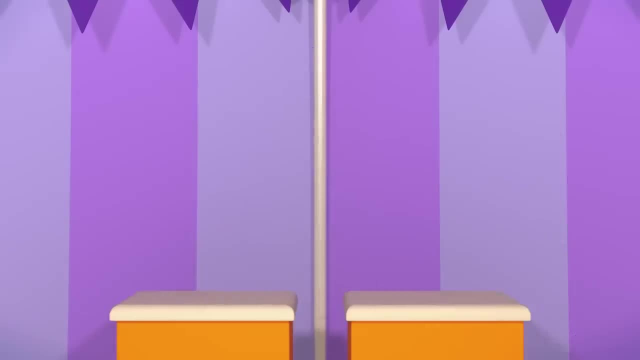 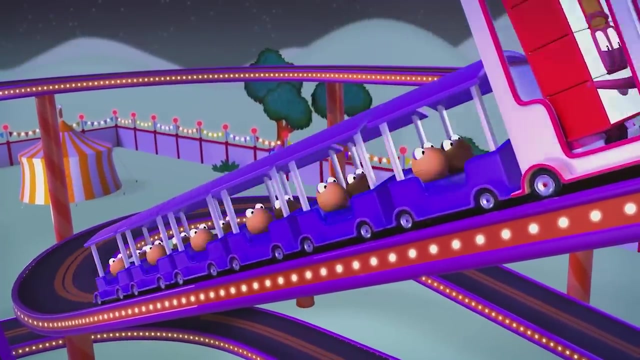 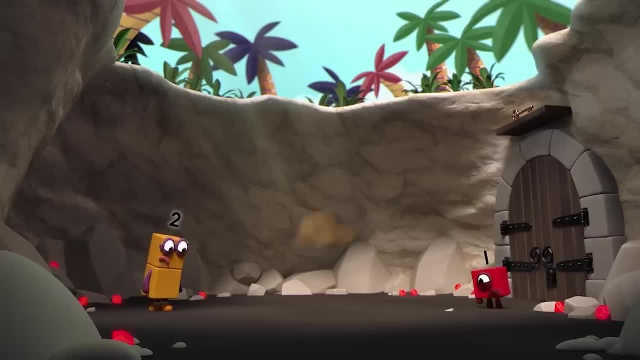 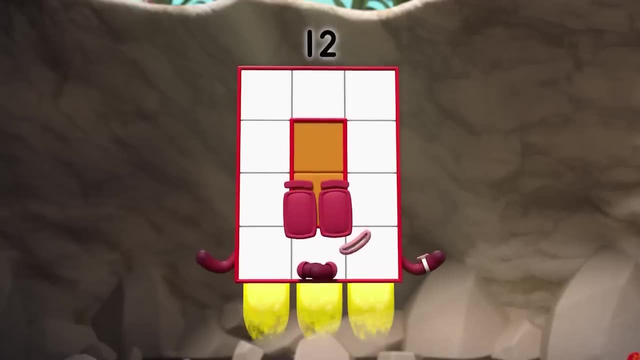 Hooray, Hooray, Hooray, Hooray, Hooray. But how do we reach it? I am the genie of the air. To win the first key, you must find all of my gems. But to make things trickier, 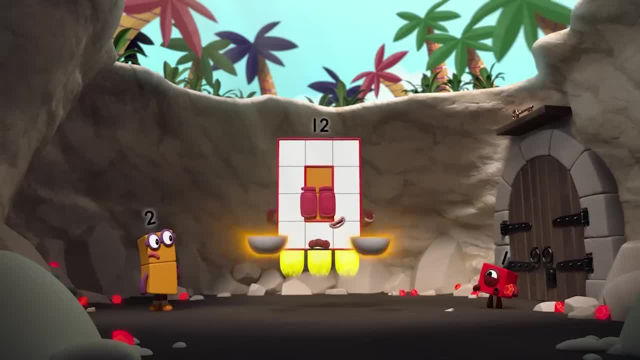 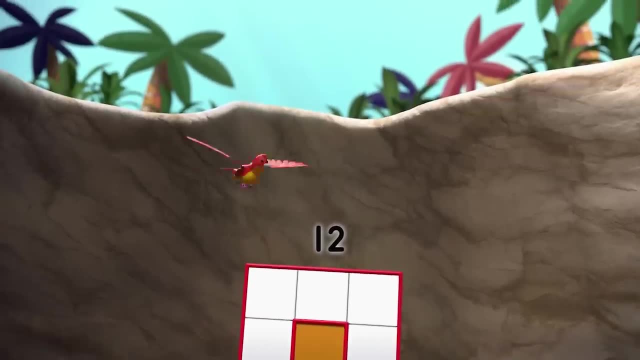 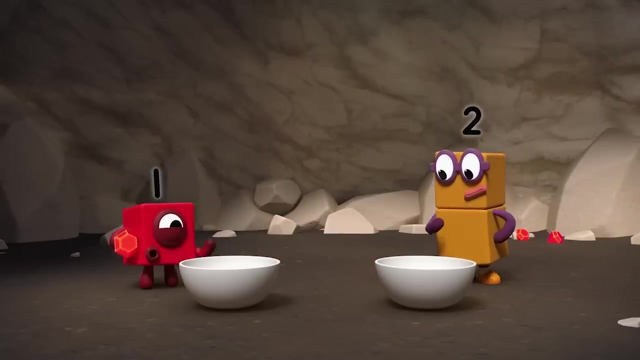 you must share the gems equally between these two bowls And hurry. when the sands of time run out. a bird will fly off with the key, Hooray, Hooray. How can we put the same number in each bowl if we don't even know how many there are? 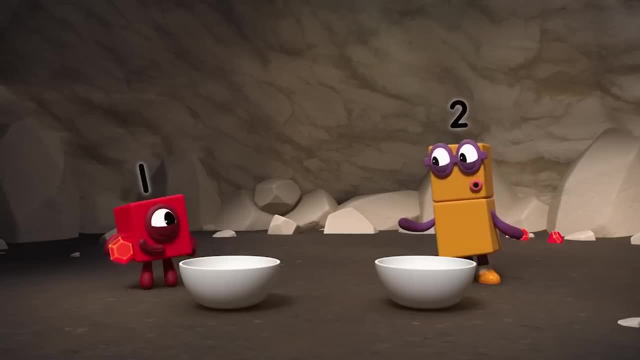 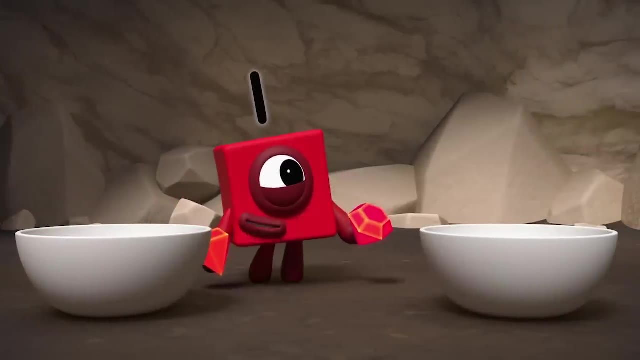 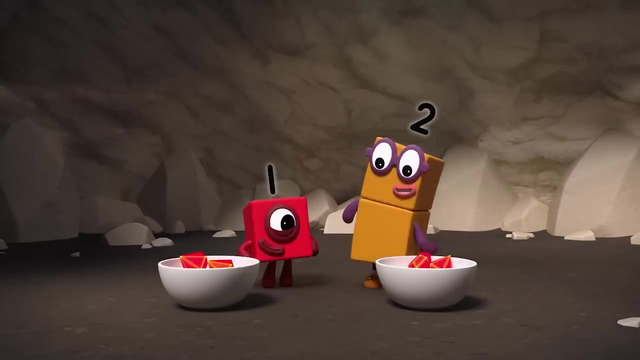 Remember how we shared the lanterns: One for you, one for me. Yes, If we put one gem into each bowl in turn, they'll always have the same number of gems: One for you, one for me, One each One for you and one for me. 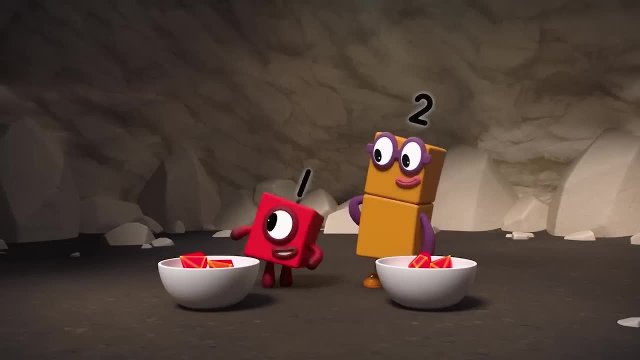 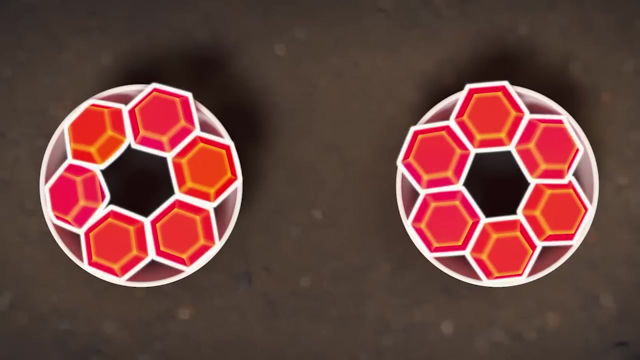 It's working. Two gems in each bowl, One for me, One for me, One for me. That's all of them. There are six gems in my bowl And six in mine. That's twelve gems altogether. That's right. 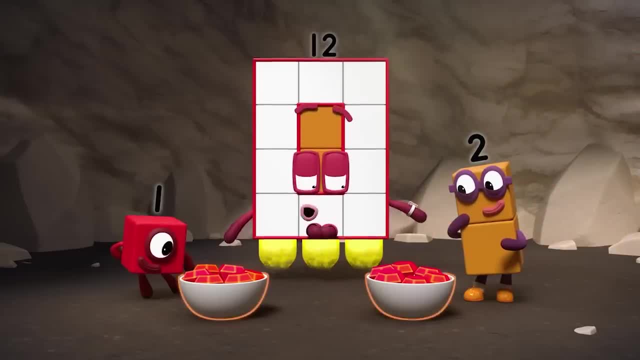 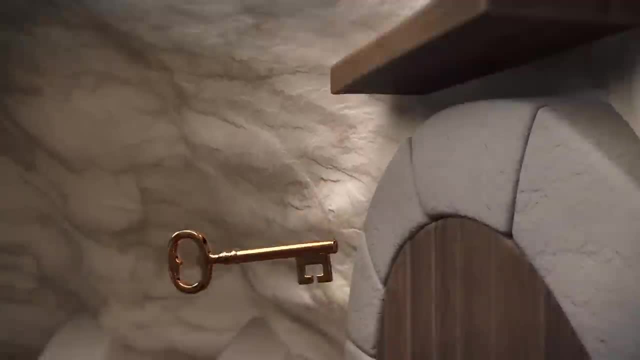 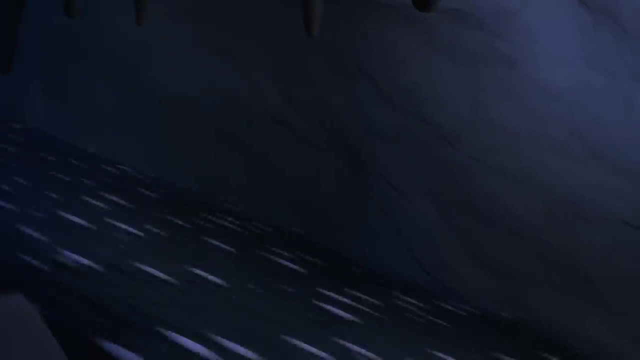 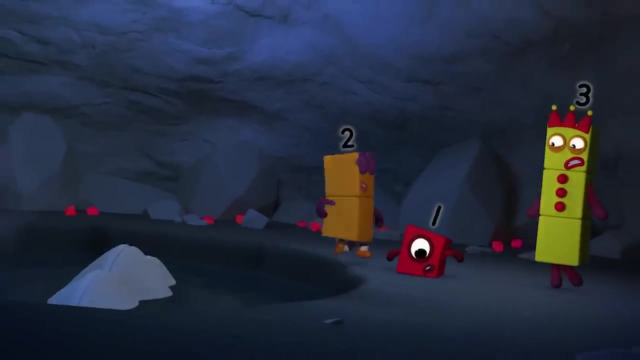 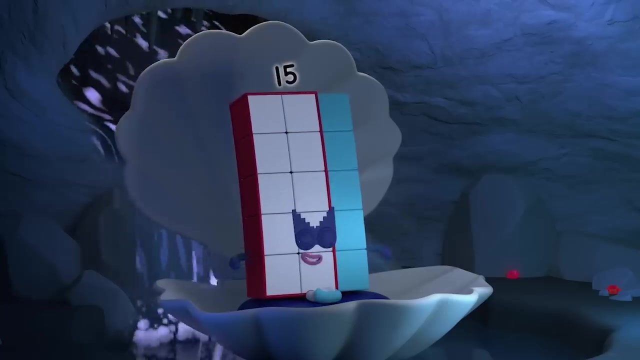 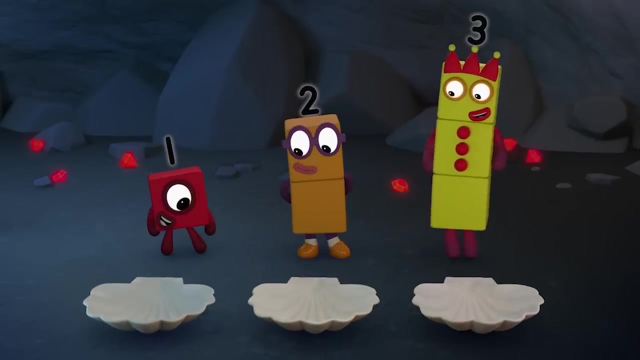 Twelve gems shared between two bowls is six in each bowl. Congratulations. There you are. I thought you'd never get here. I am the genie of water. Your next challenge is to share my fifteen watery gems between these three shells, So each shell has the same number of gems. 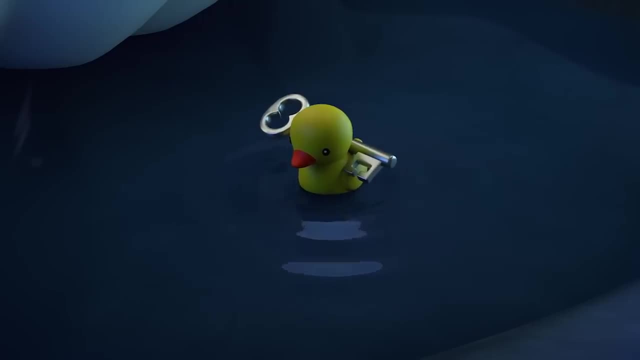 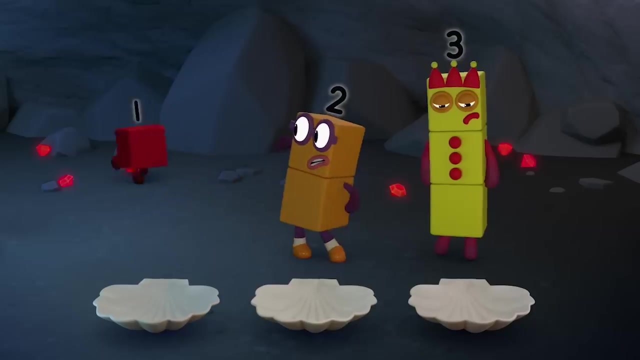 The next key: Share the gems. Share the gems before the waters run dry or the key will be sucked down. the bottomless plug hole. Quick One gem at a time. No, no, no, That's too slow. Let's get three at a time. 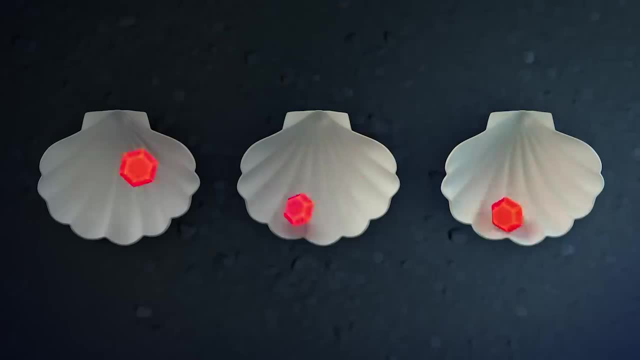 Three shells, three gems, One gem in each shell. Good thinking, three, Three shells, three gems, Two gems in each shell. Each time there's one more in each shell, Three more and three more, And that's all of them.